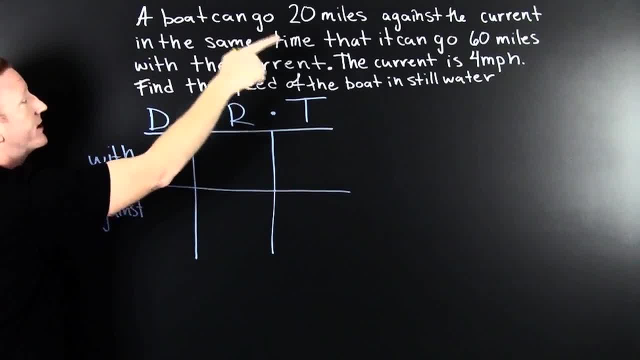 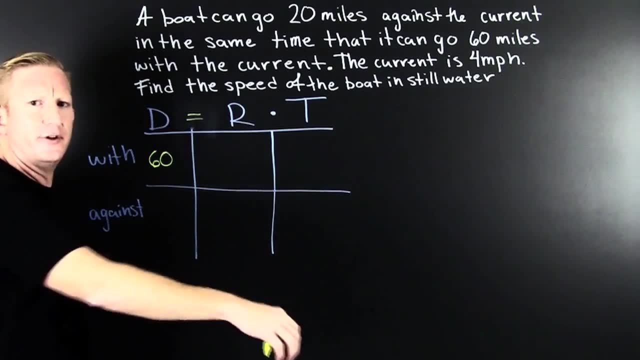 With the current. how far does this boat go With the current? it goes 60 miles With against the current. I know you've been in the water before and you try to walk against the current. You don't go as fast as when you turn around. 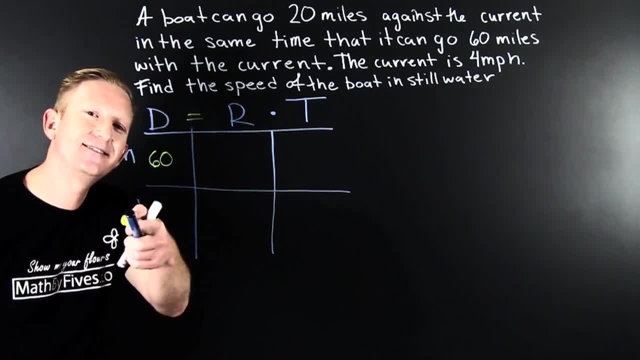 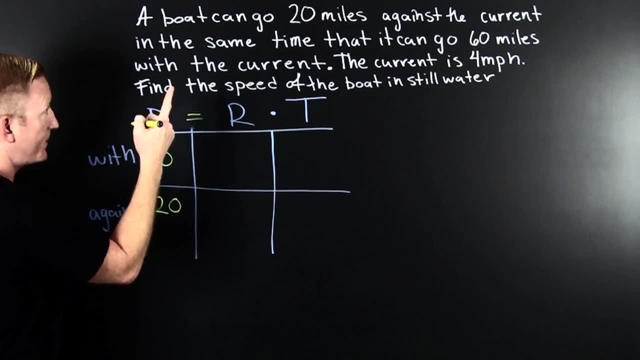 And have all the wind to your back Or water to your back, And this is also how those airplane problems go too. So then I'm down here. Against the current, it goes 20 miles. That's what that guy says up there. 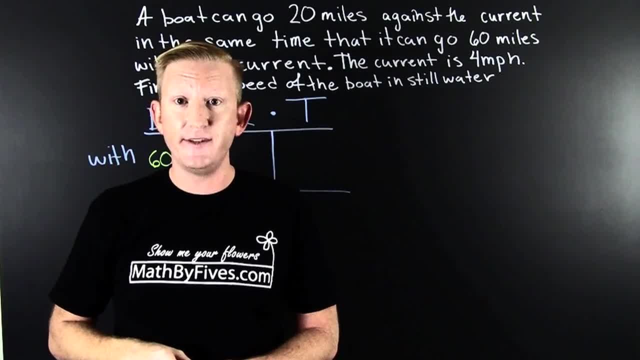 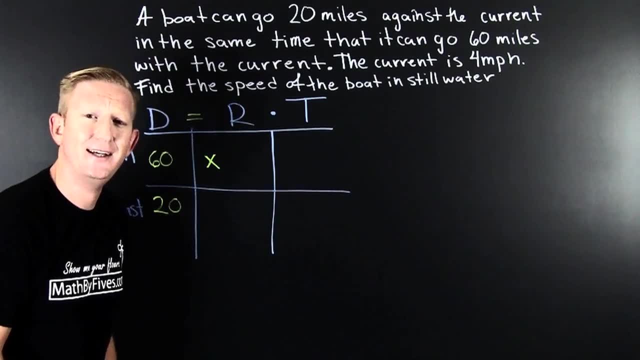 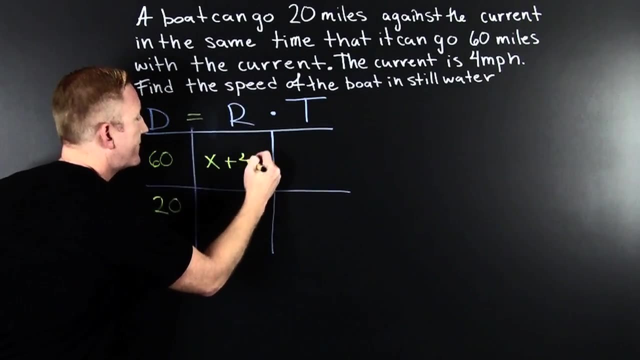 The rates. Oh boy, We're trying to find the rate of this boat. We don't know, So let's call it x, Alright, With the current. is the boat aided or hindered by the current? It's aided, It goes faster. So this is x plus 4.. 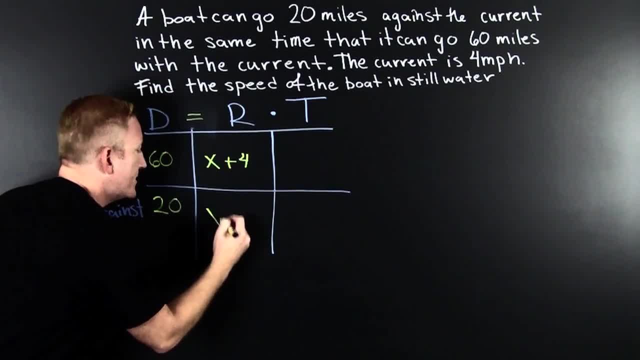 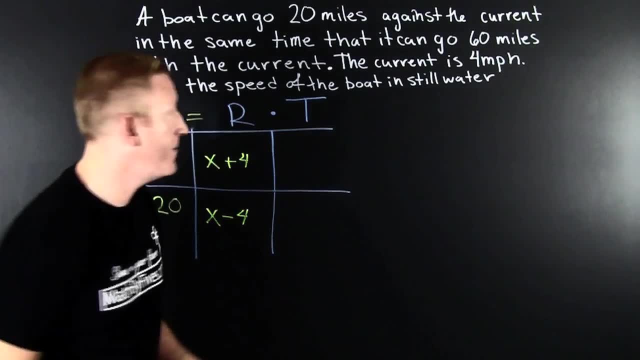 Sure, Now when you're going against the current, it works against you. So no matter how fast you're going, subtract 4 from it. Alright, So my math does have this relationship. The rate times the time is the distance. 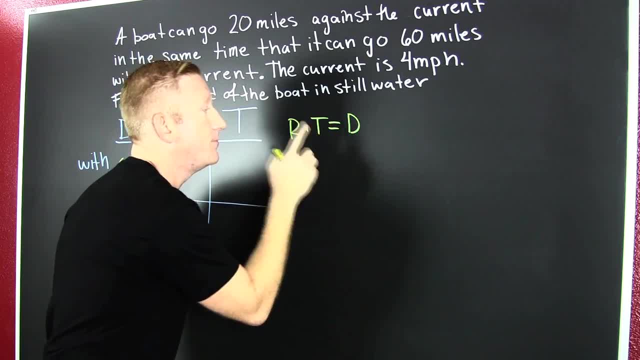 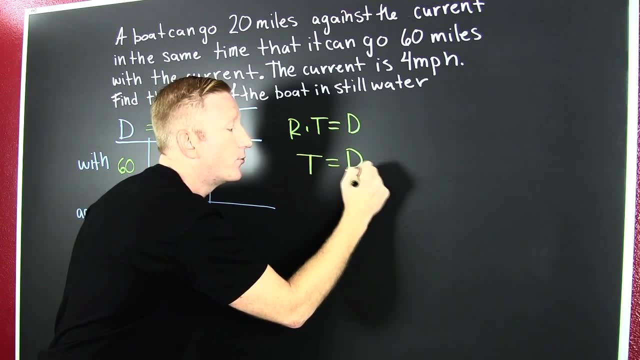 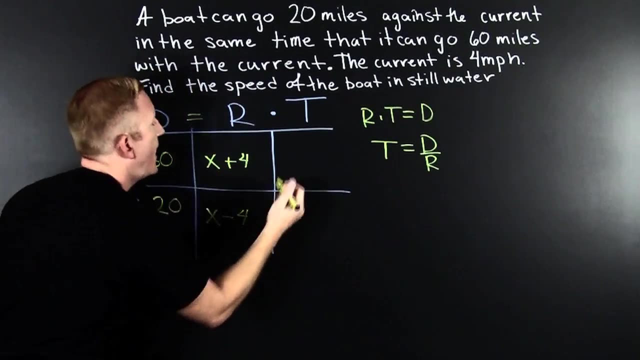 And what do we want? We want to find that time. So we're going to divide both sides by the rate, And our time is going to be our distance divided by our rate, And that's what's happening right now. So I'm going to take that distance and divide it by that rate. 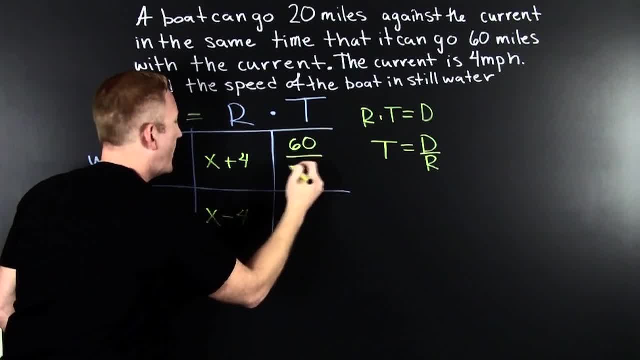 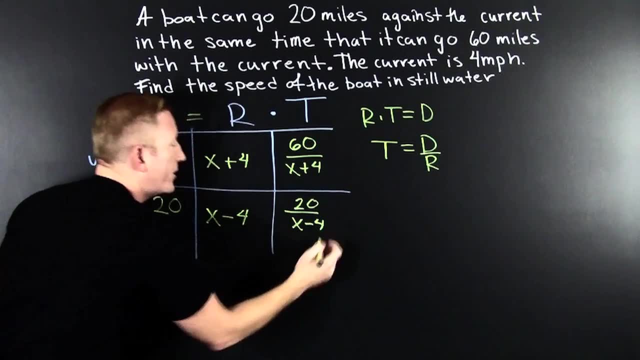 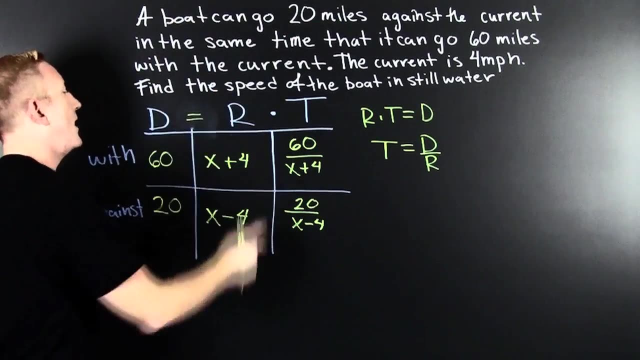 And when I do, I'm going to have that 60 divided by that x plus 4.. And then down there I'm going to have that 20 divided by x minus 4.. And now we explore what the problem says. The boat can go 20 miles against the current in the same time. 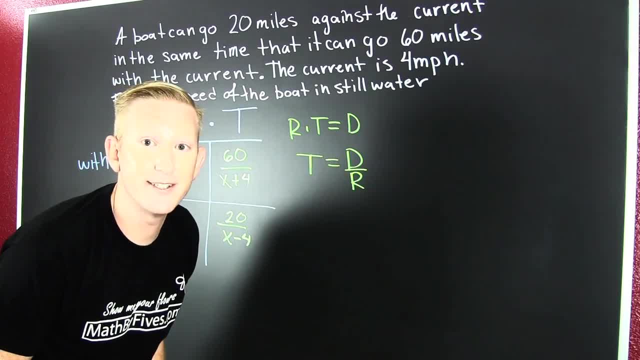 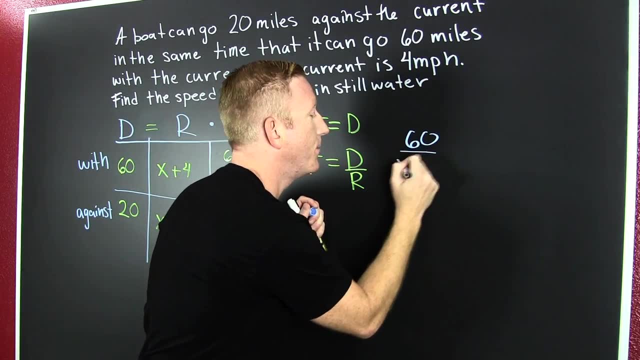 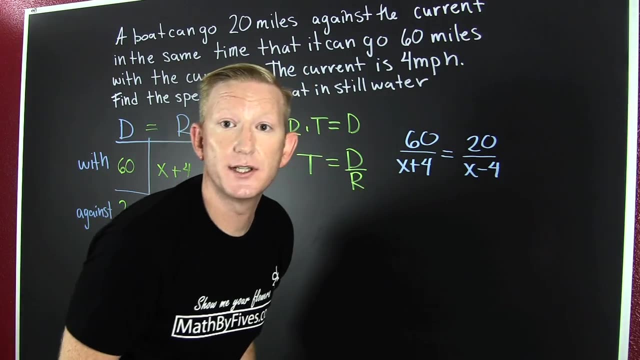 If the times are the same, then that means the times are the same, And we're going to set it up like that. It's going to be: 60 is to x plus 4 as 20 is to x minus 4.. And then we're going to use a little cross multiplication. 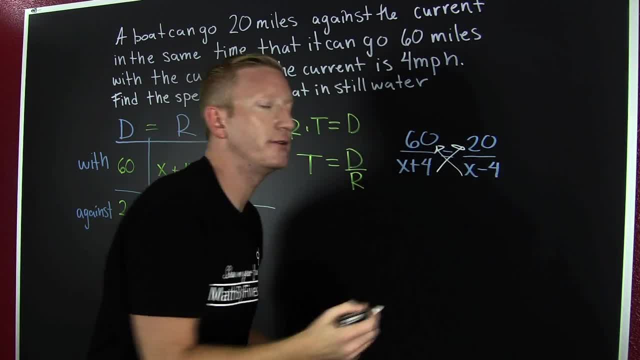 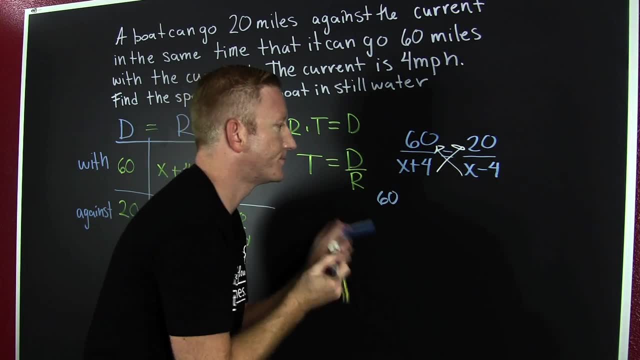 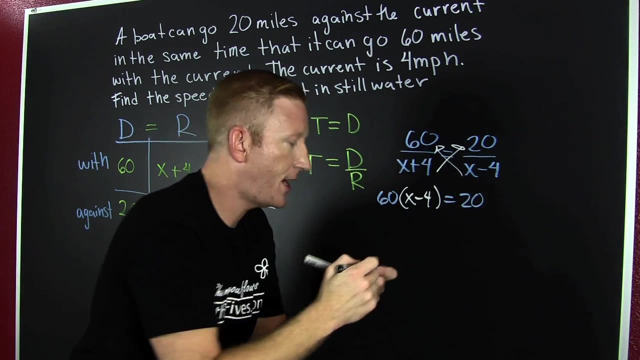 A little bit of this, a little bit of that. Clearing those fractions, multiplying both sides by the common denominator, if that's how you want to see it. So then I'm going to have 60 times an x minus 4, that's going to be equal to 20 times.